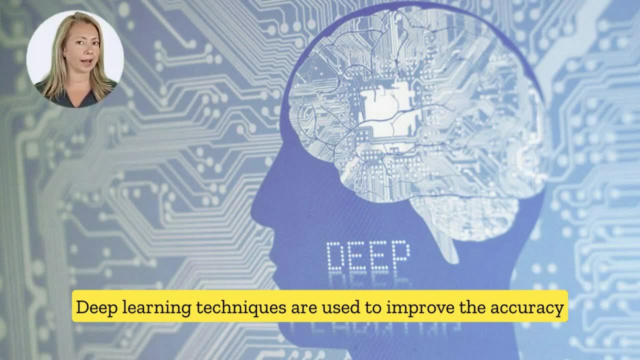 Deep learning techniques are used to improve the accuracy and efficiency of computer vision systems. These techniques use neural networks with multiple layers to learn and recognize patterns in images and videos. Examples include Convolutional Neural Networks, Recurrent Neural Networks and Generative Adversarial Networks. 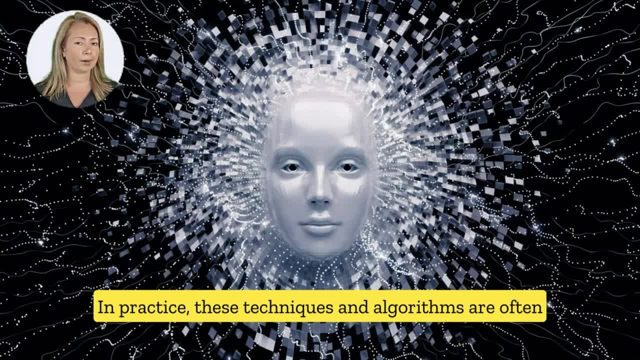 In practice, these techniques and algorithms are often used in combination to analyze images and videos. For example, image processing techniques are often used to pre-process images and extract features which are then used by object recognition and facial recognition algorithms to detect and classify objects and faces. 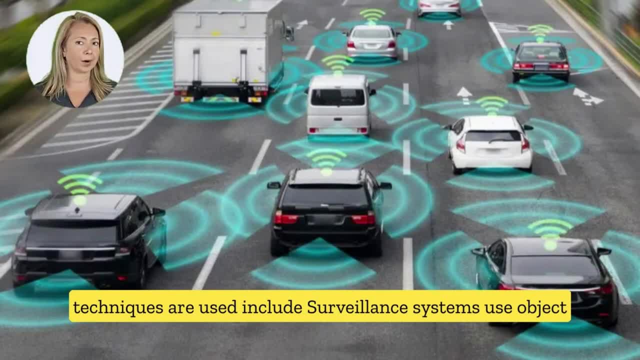 Some of the real-world examples where these techniques are used include: Surveillance systems: use object recognition algorithms to detect and track people, cars and other objects in the camera footage. Autonomous vehicles: use object recognition algorithms to detect and identify people. Autonomous vehicles: use object recognition algorithms to detect and identify cars, pedestrians and traffic signs to navigate. 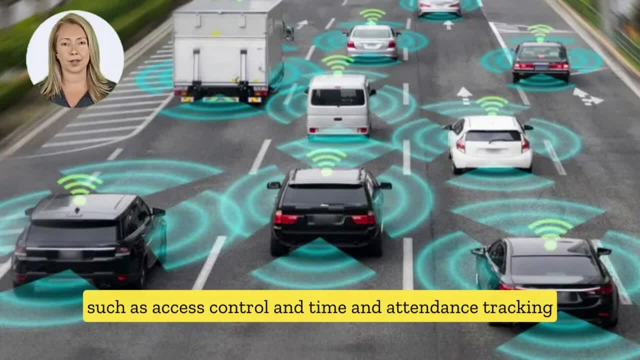 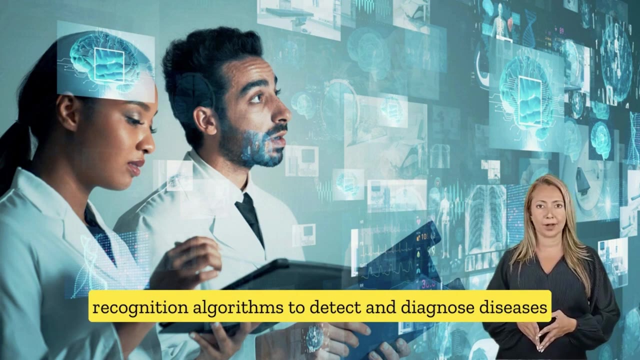 Facial recognition systems are used in security applications such as access control and time and attendance tracking, as well as in marketing, to identify and track customers in retail stores or other public spaces. Medical imaging systems use image processing and object recognition algorithms to detect and diagnose diseases and injuries. 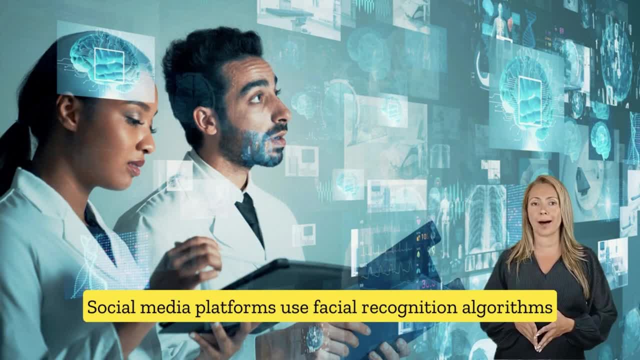 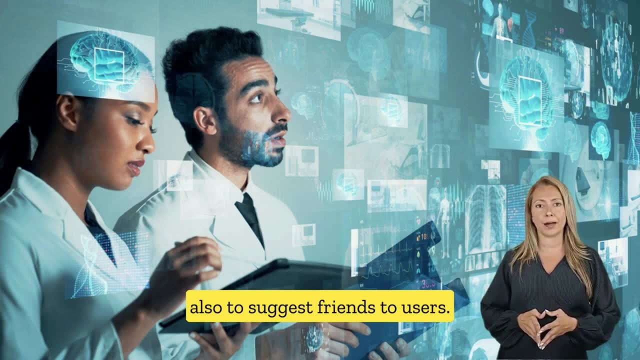 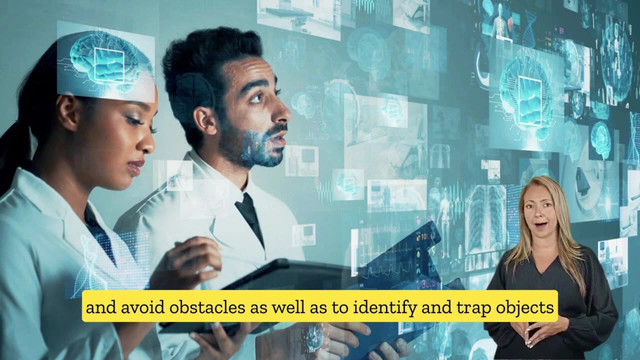 such as tumors in CT scans or X-rays. Social media platforms use facial recognition algorithms to automatically tag individuals in photos and also to suggest friends to users'. robotics and drones use object recognition to detect and avoid obstacles, as well as to identify and track objects of interest. 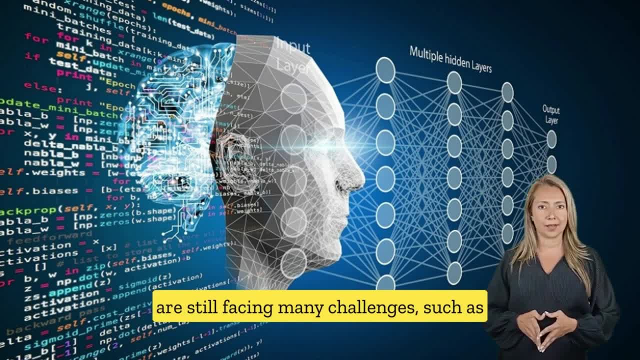 These techniques are not perfect and they are still facing many challenges, such as dealing with variations in lighting, pose and occlusion, and generalizing to new scenarios. However, with the advancements in technology, these techniques are becoming more accurate, efficient and robust. 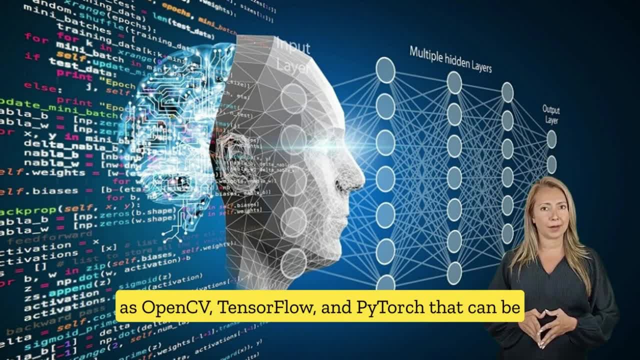 There are several popular computer vision libraries, such as OpenCV, TensorFlow and PyTorch, that can be used to process image data and gain insights. Here's an overview of how to use these libraries. OpenCV Open Source Computer Vision Library is a library of programming functions mainly aimed at real-time computer vision. 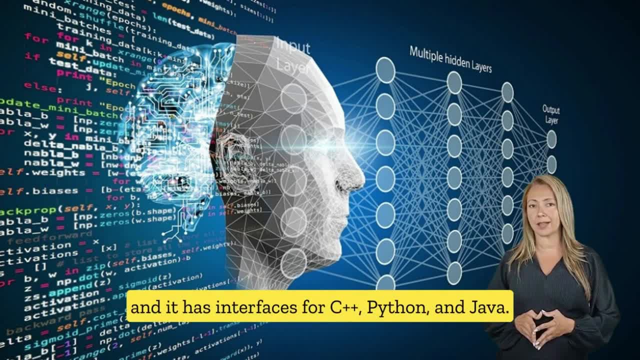 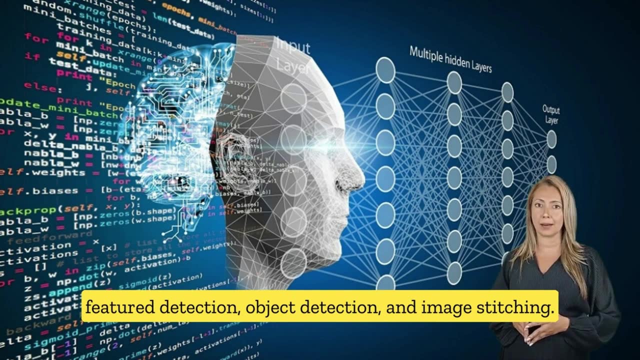 It is open source and free to use, and it has interfaces for C++, Python and Java. OpenCV provides a wide range of image processing and computer vision functions, including image filtering, feature detection, object detection and image stitching. To use OpenCV in Python: 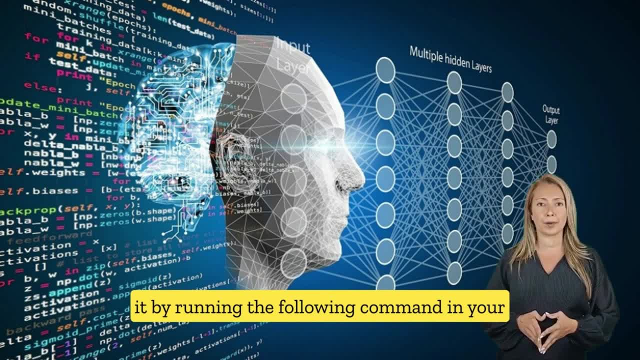 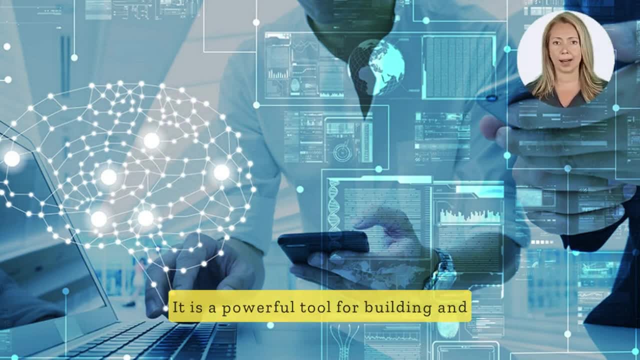 you can install it by running the following command in your terminal Pick: Install OpenPython. TensorFlow is an open source machine learning library developed by Google. It is a powerful tool for building and deploying machine learning models, and it has a built-in support for computer vision tasks. 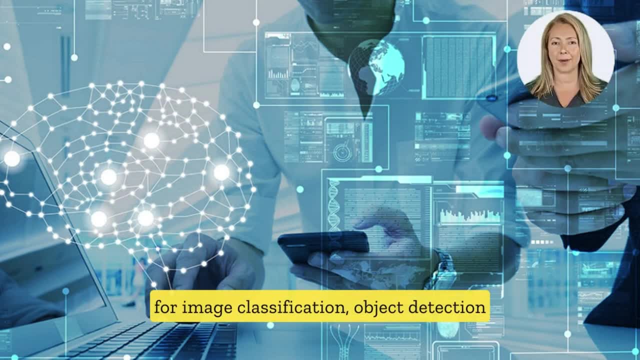 TensorFlow provides a wide range of pre-trained models for image classification, object detection and image segmentation which can be fine-tuned for specific tasks. To use TensorFlow in Python, you can install it by running the following command in your terminal pip: install tensorflow. 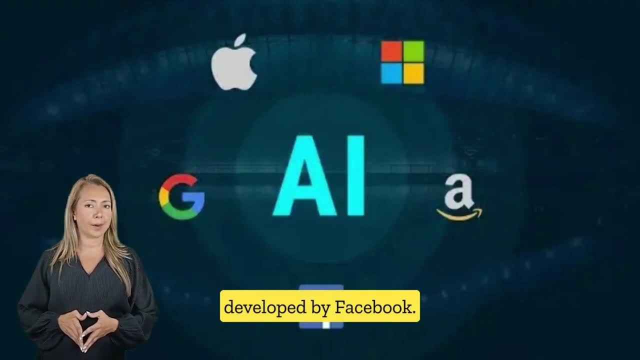 ByTorch is an open-source machine learning library developed by Facebook. It is similar to TensorFlow in terms of functionality, but it is more developer-friendly and has a more Pythonic API. ByTorch provides a wide range of pre-trained models for image classification. 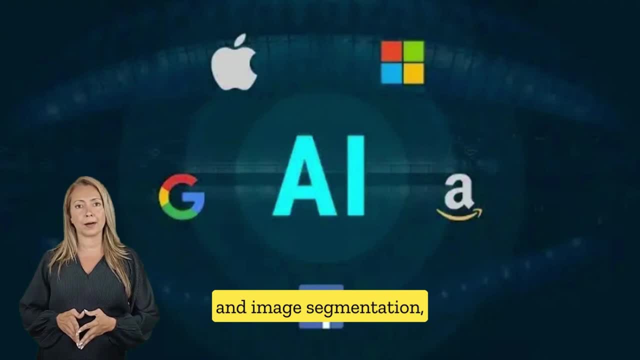 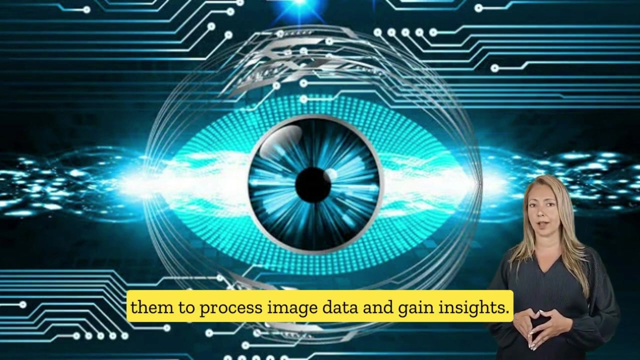 object detection and image segmentation, which can be fine-tuned for specific tasks. To use PyTorch in Python, you can install it by running the following command in your terminal: pip: install tort. Once you have installed these libraries, you can start using them to process image data and gain insights. 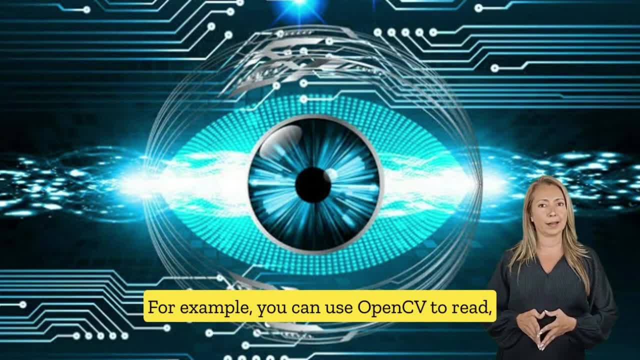 For example, you can use OpenCV to read, display and write images, perform image filtering and feature detection, and use TensorFlow or PyTorch to perform image classification, object detection and image segmentation. It's worth noting that these libraries are complex and it's recommended to have a good understanding of programming and computer vision concepts.